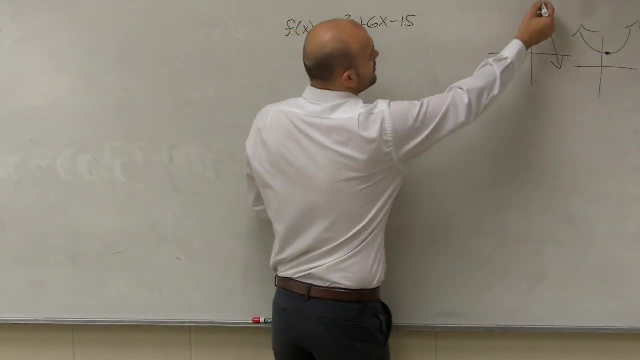 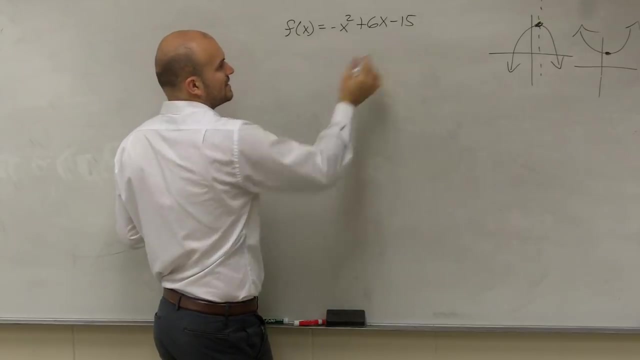 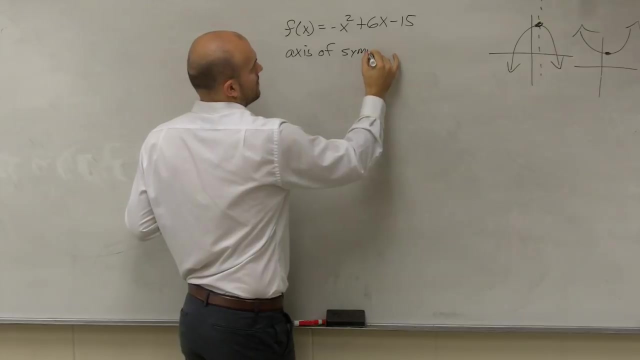 Vertex, right. So how did we find the vertex? Well, what we remembered was the vertex went through the axis of symmetry. So the first thing I want to do is determine what is the axis of symmetry. So the axis of symmetry is, if you guys remember the formula, 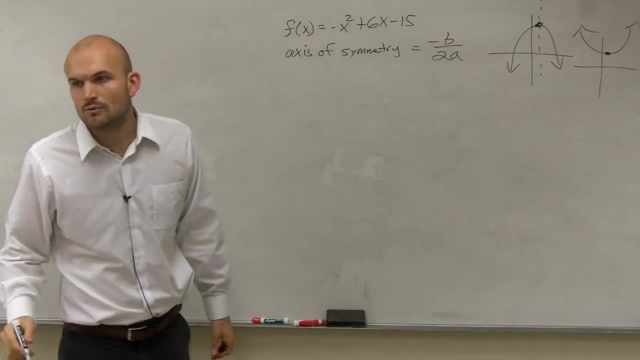 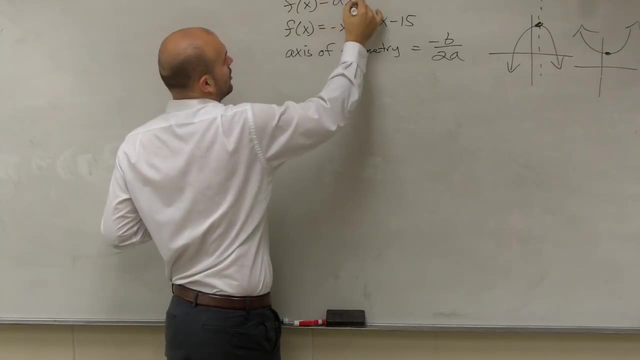 it's going to be the opposite of B divided by 2A. Now what was B and A? Remember all quadratics? all quadratic equations come in the form AX squared plus BX plus C, where A, B and C are real numbers, where A cannot equal zero. 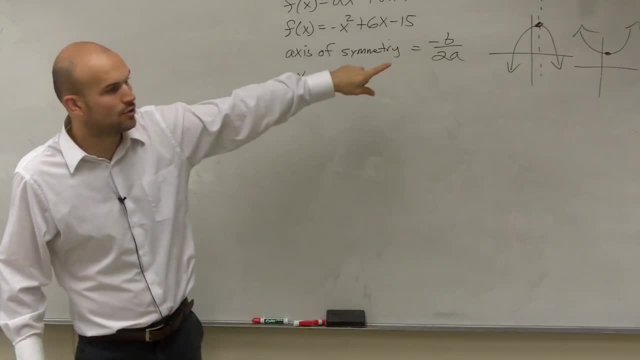 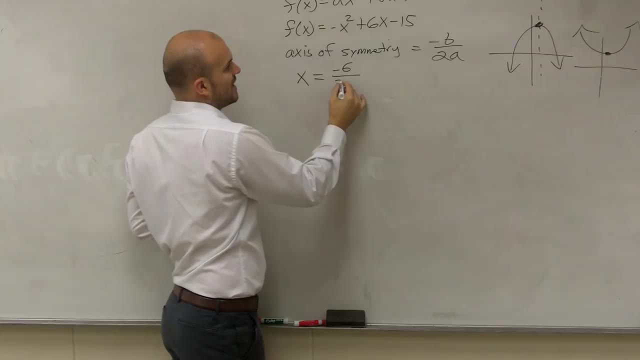 So in this formula I say, the axis of symmetry or the X coordinate of my vertex is going to equal. X, equals opposite of B, which in this case is a negative 6, divided by 2 times negative 6.. Negative 1, where B is negative 6 and A is negative 1.. 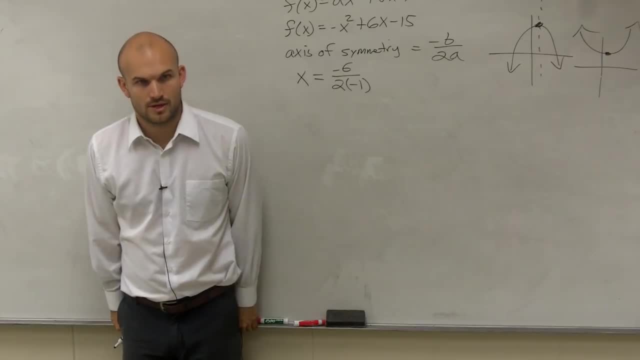 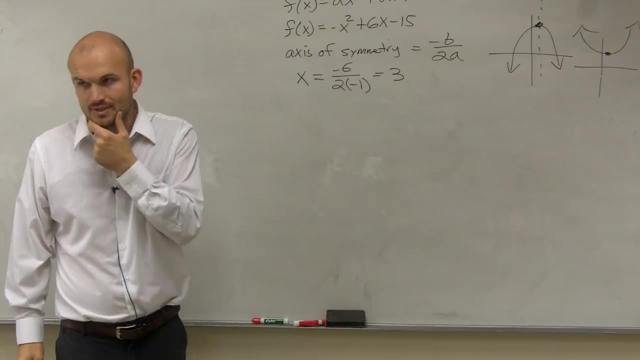 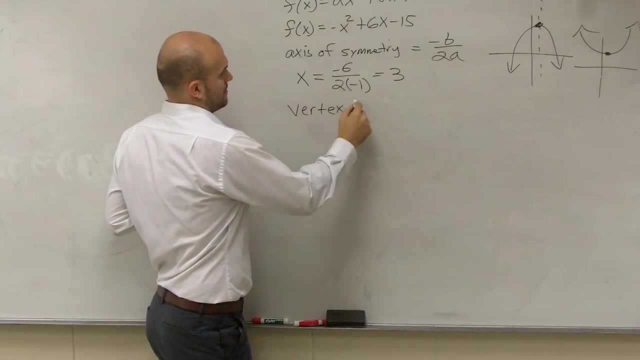 Anybody have any questions? up to this point, No, So therefore I figure this out and I get the X coordinate equals 3.. Right, So that means my X coordinate is equal to 3 and my vertex So it's 3 comma. what? 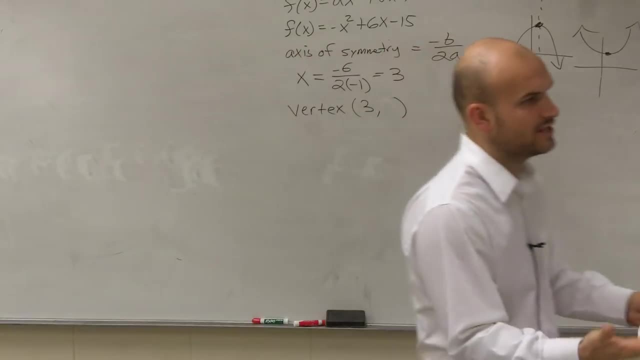 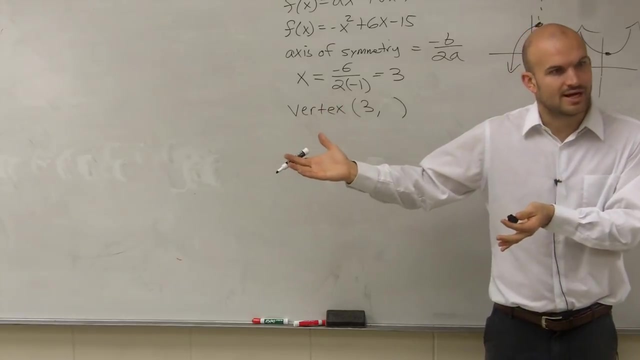 So, ladies and gentlemen, in a function, if you know one value, if you know the input or the X, how do you find the Y value? Yes, Sean, You plug it in for your X value, right, We know the X. 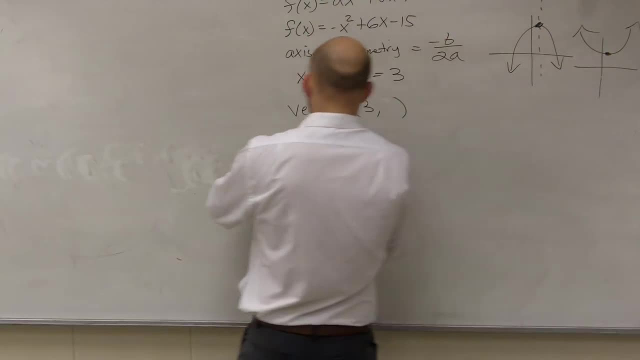 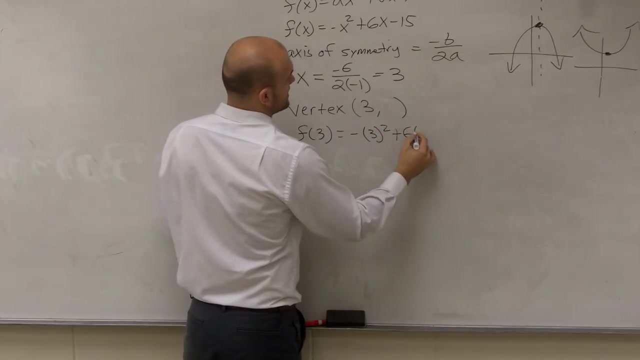 We need to figure out the F of X or the output value. So what I do then is I take F of 3, and I get negative 3 squared plus 6 times 3 minus 15.. This becomes a negative 9 plus 18 minus 15,. 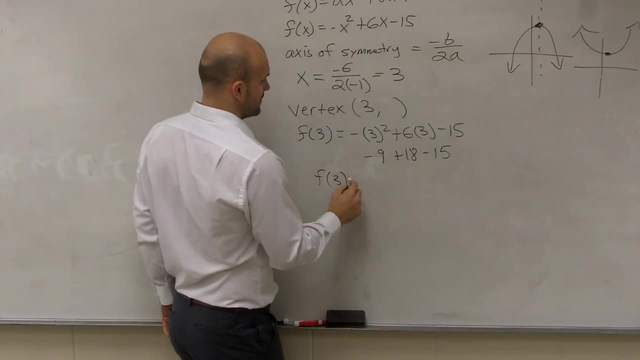 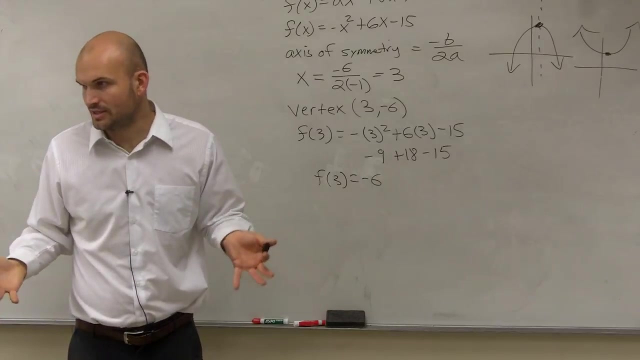 which ends up giving me F of 3 equals negative 6.. So if I was going to plot this, ladies and gentlemen, I don't really know exactly what this graph looks like, but I know right now that I have a point. 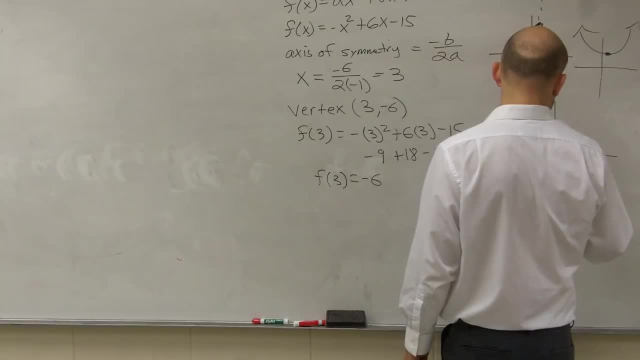 My vertex is at 3, negative 6.. 1,, 2, 3, 1, 2, 3,, 4, 5, 6.. Okay, So my point's right there. Now what I need to do is determine. 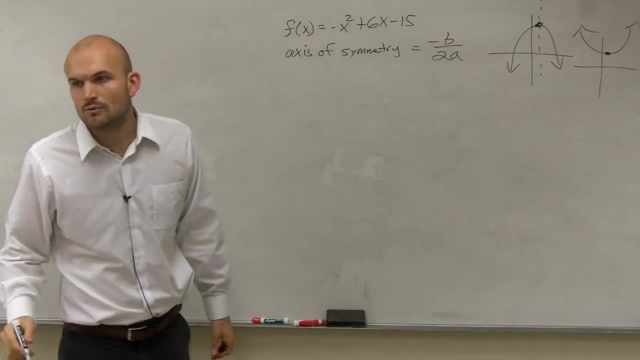 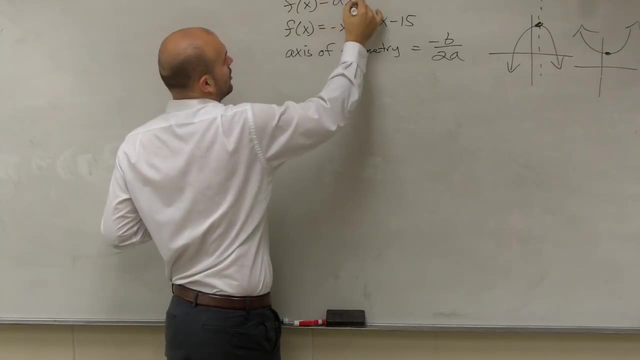 it's going to be the opposite of B divided by 2A. Now what was B and A? Remember all quadratics? all quadratic equations come in the form AX squared plus BX plus C, where A, B and C are real numbers, where A cannot equal zero. 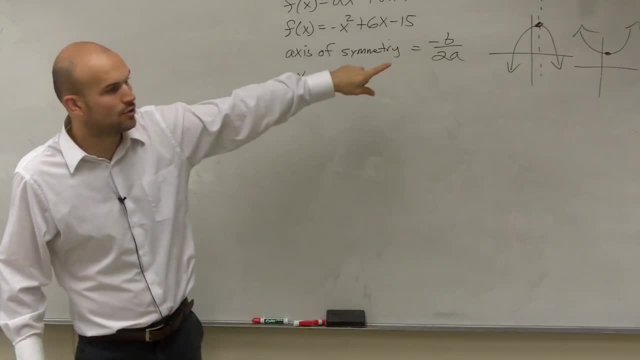 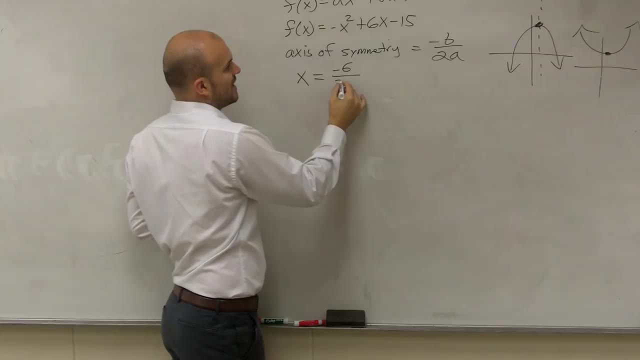 So in this formula I say, the axis of symmetry or the X coordinate of my vertex is going to equal. X, equals opposite of B, which in this case is a negative 6, divided by 2 times negative 6.. Negative 1, where B is negative 6 and A is negative 1.. 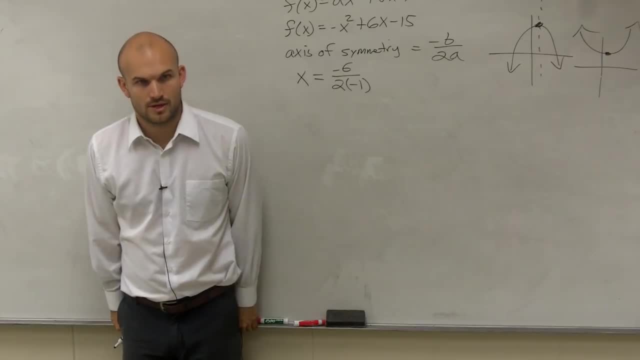 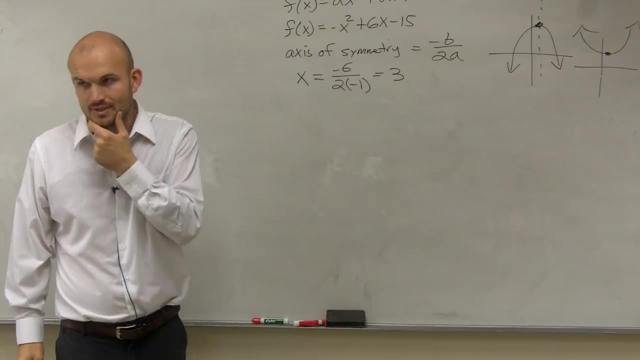 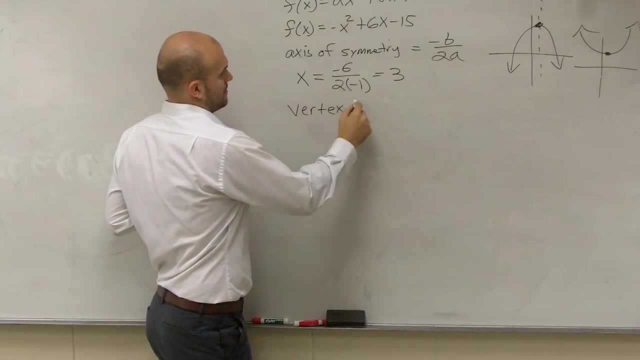 Anybody have any questions? up to this point, No, So therefore I figure this out and I get the X coordinate equals 3.. Right, So that means my X coordinate is equal to 3 and my vertex So it's 3 comma. what? 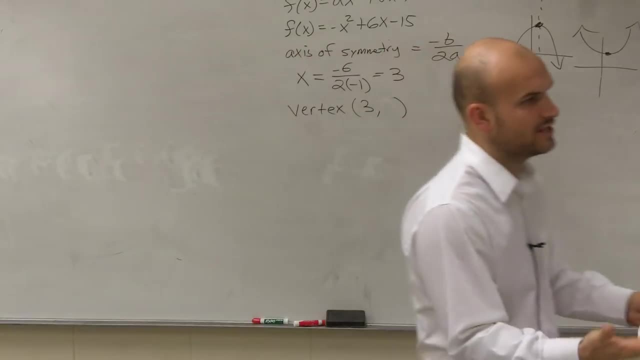 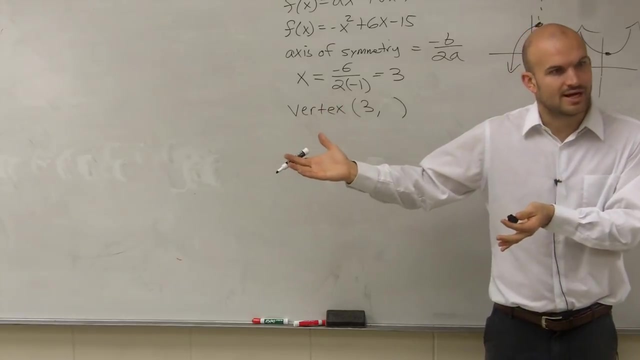 So, ladies and gentlemen, in a function, if you know one value, if you know the input or the X, how do you find the Y value? Yes, Sean, You plug it in for your X value, right, We know the X. 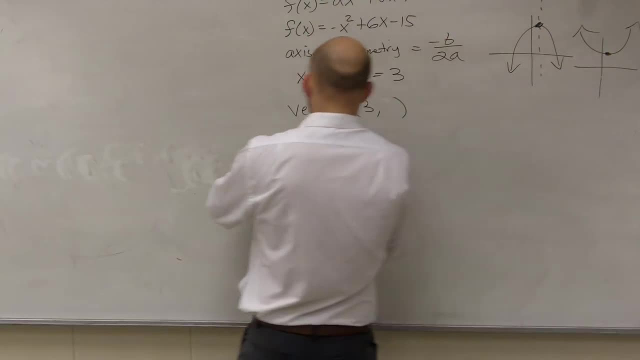 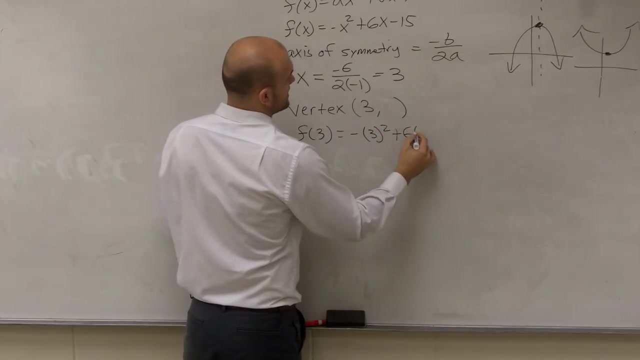 We need to figure out the F of X or the output value. So what I do then is I take F of 3, and I get negative 3 squared plus 6 times 3 minus 15.. This becomes a negative 9 plus 18 minus 15,. 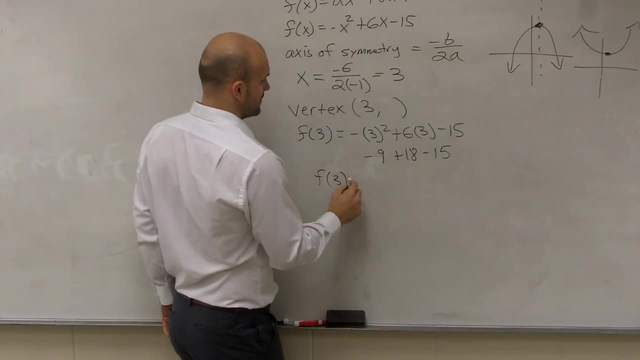 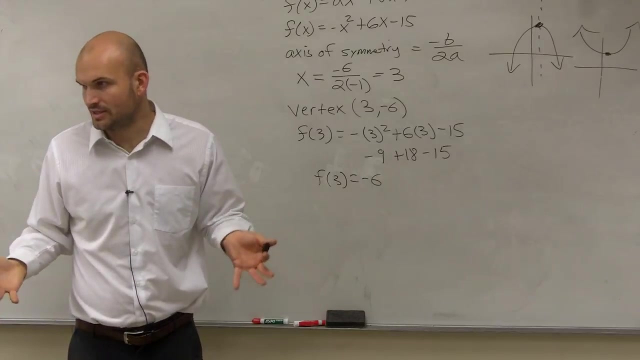 which ends up giving me F of 3 equals negative 6.. So if I was going to plot this, ladies and gentlemen, I don't really know exactly what this graph looks like, but I know right now that I have a point. 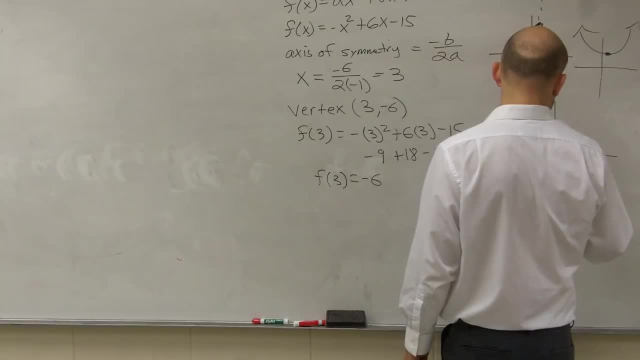 My vertex is at 3, negative 6.. 1,, 2, 3, 1, 2, 3,, 4, 5, 6.. Okay, So my point's right there. Now what I need to do is determine. 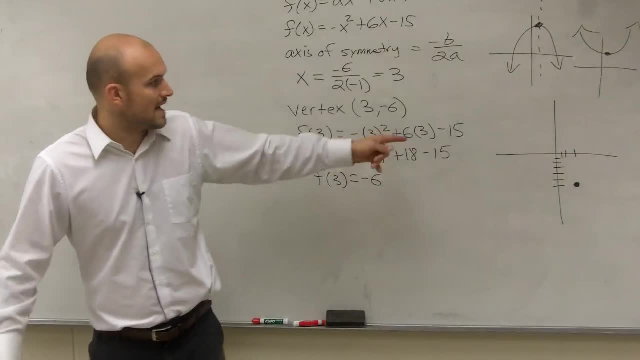 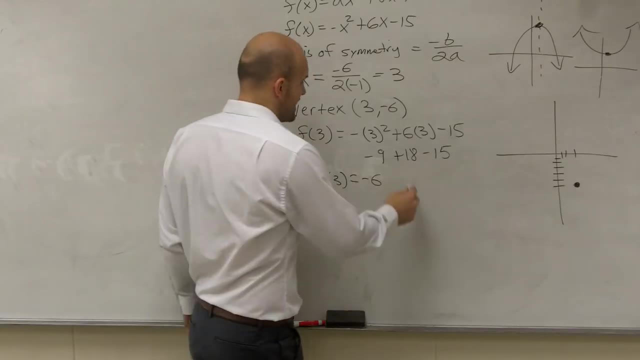 is it a maximum or a minimum? What is that point? Is that the maximum Or is that the minimum of the graph? So remember, there was a rule, There was a test we looked at And that test said: whenever you had A was less than 1, I'm sorry, 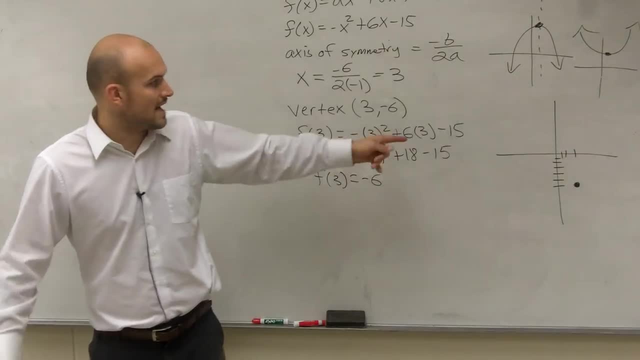 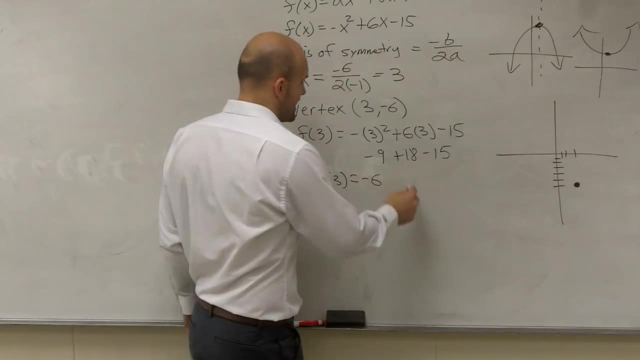 is it a maximum or a minimum? What is that point? Is that the maximum Or is that the minimum of the graph? So remember there was a rule, There was a test we looked at And that test said: whenever you had A was less than 1.. 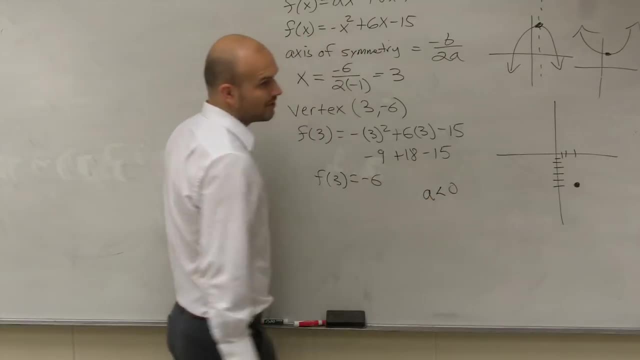 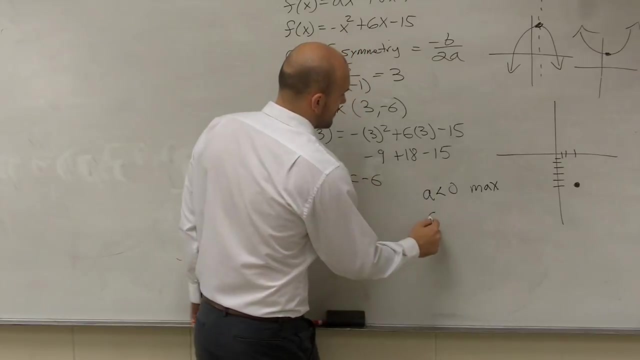 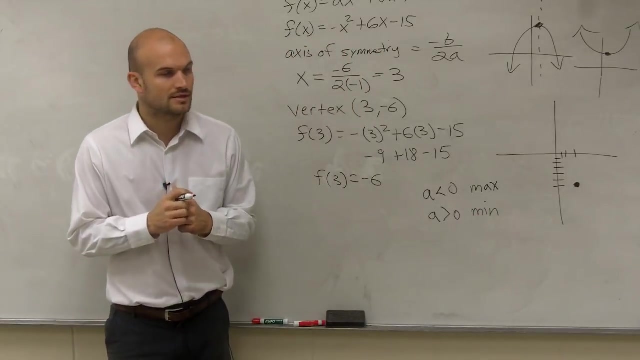 I'm sorry. When A was less than 0, that means you had a maximum point, And when A was greater than 0, that means your vertex was minimum Was your minimum point. So we look at this and we write. 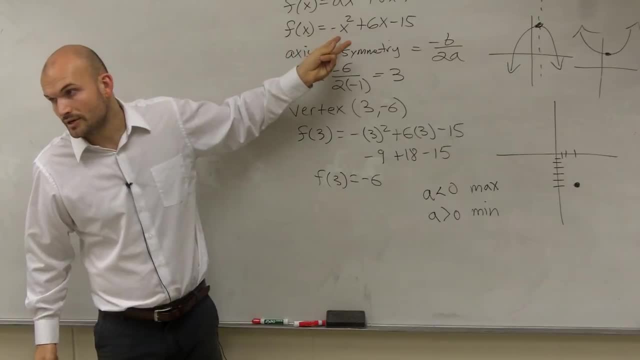 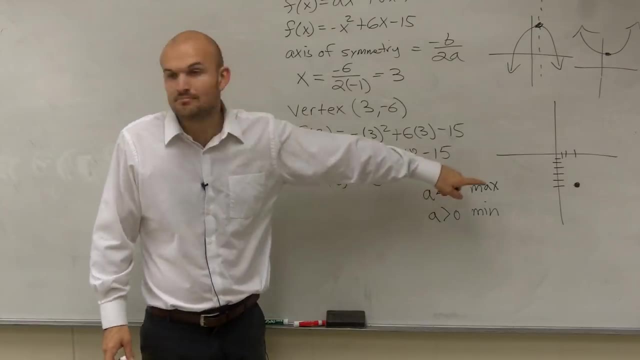 down. we say: all right, what was my A? My A is negative, 1, correct, So is A greater than or less than Less than So. therefore, that means that's a maximum point, Right? So my graph's going to look something like this: 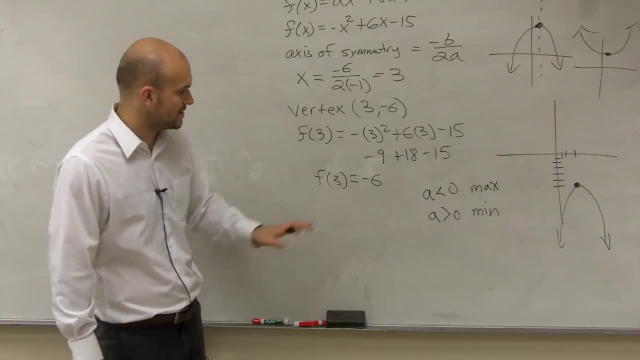 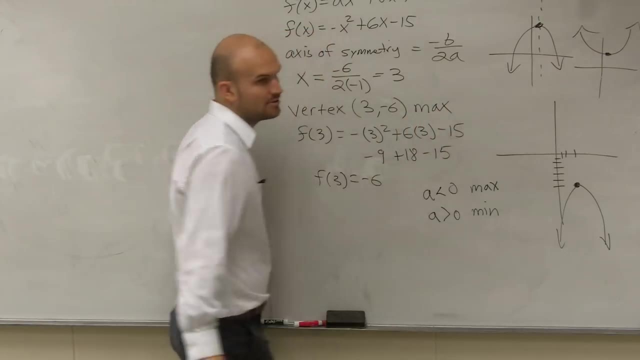 All right, I'm just going to. we're not going to work on sketching it right now. We'll do table values later. So my maximum point looks like that. So we could say: that's my vertex, which is a maximum point. 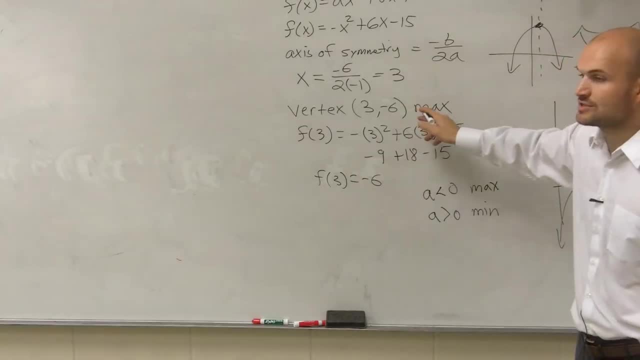 So that's what you guys should have wrote for your maximum point. That is my vertex, which is a maximum point because the graph opens down because of this rule that we worked on. Then the next thing that got students very confused was the. 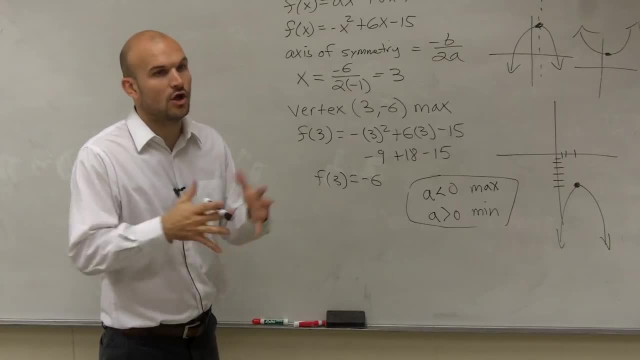 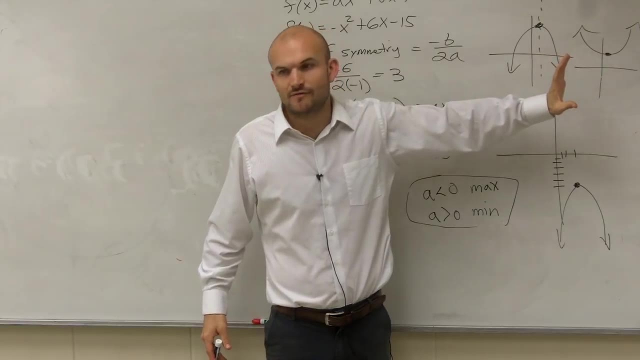 domain and range. Remember, the domain is the set of all X values that are part of your graph. Ladies and gentlemen, look at these two parabolas, All right, And think about any parabola you've ever graphed or looked at. 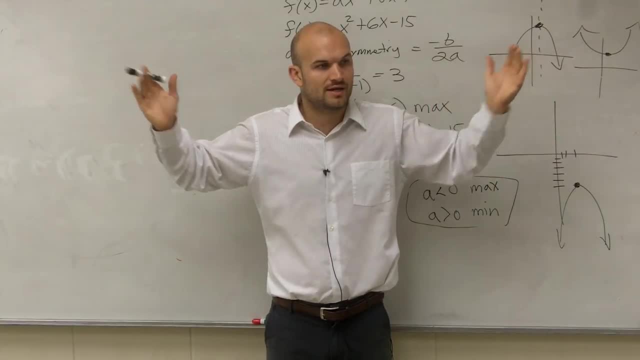 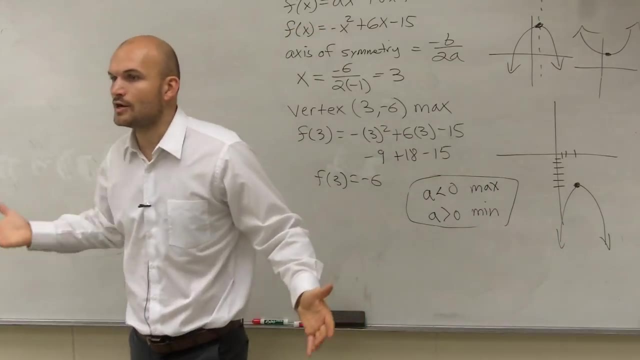 These parabolas are going to infinitely just keep on getting wider and wider. right As they go up, they're going to keep going. They're going to keep on expanding As they go down, they just keep on getting wider. So eventually they are going to encompass every single X value. 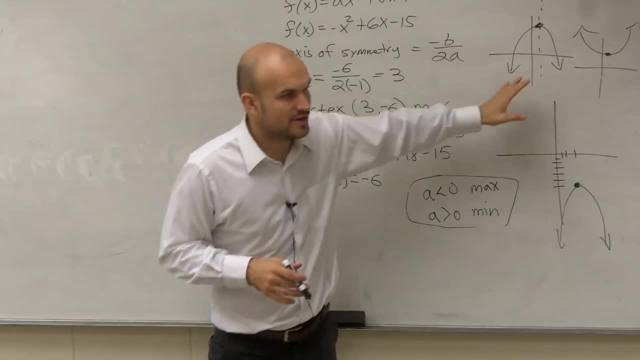 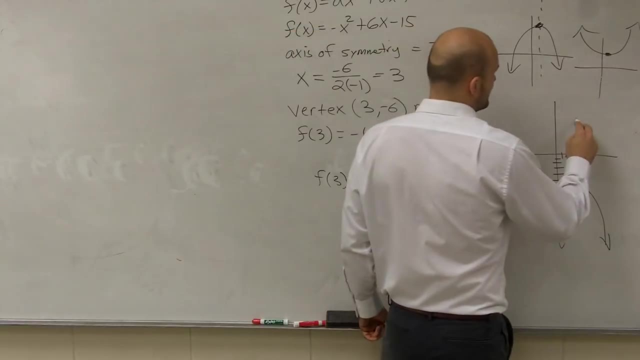 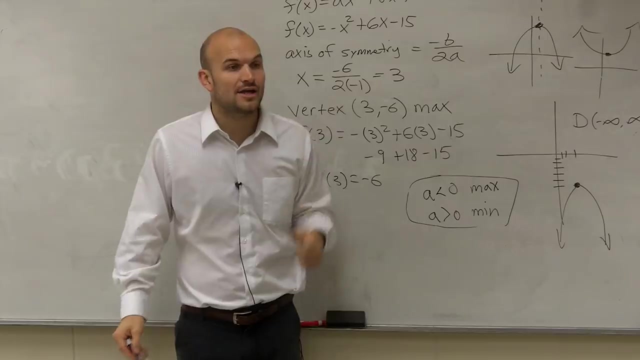 that we have in the number system, every single one. So therefore, the domain for a quadratic without any constraints is going to be all real numbers. So your domain is going to go from negative infinity to infinity. Pick any value to be X. Emma, give me a value for X. 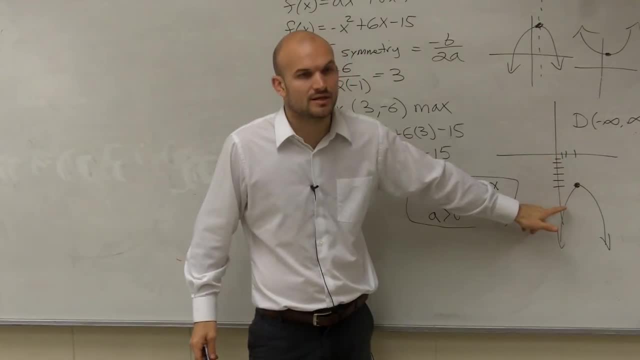 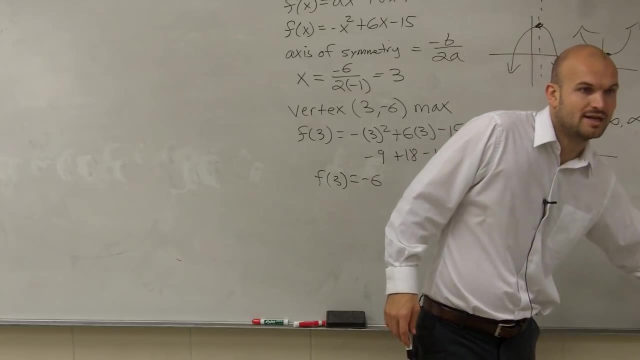 Two. Two Is two a value. Yes, It's right there. Give me another one, Eighteen. Eighteen Probably be over here, right, But when you go down, will this graph eventually have a coordinate at 18?? 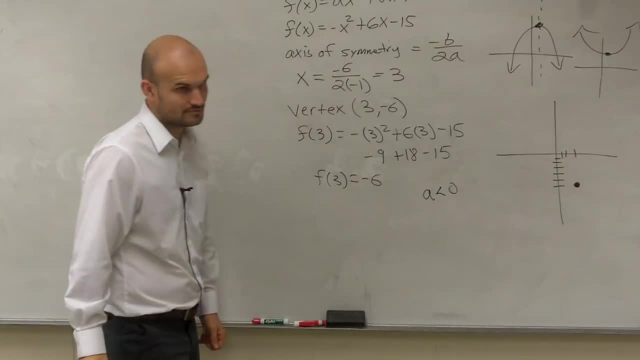 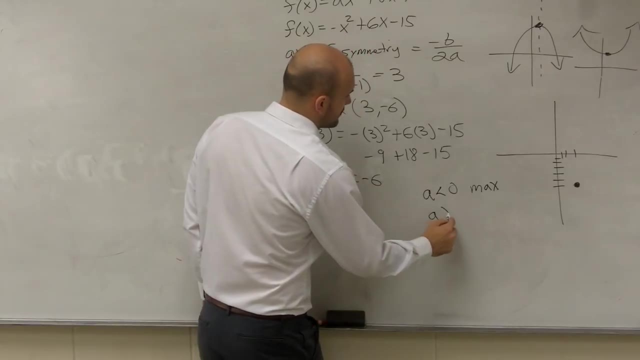 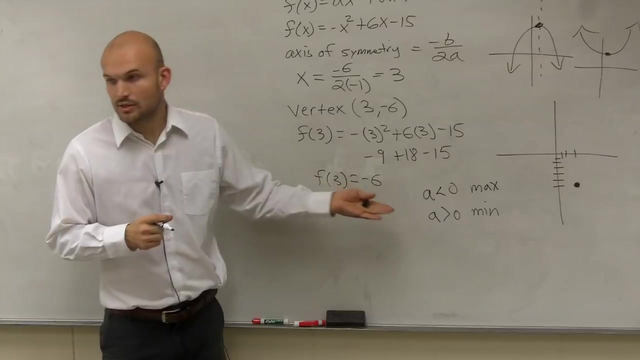 when A was less than 0, that means you had a maximum point. And when A was greater than 0,, that means your vertex was minimum Was your minimum point. So we look at this and we write down. we say, all right, what was my A? 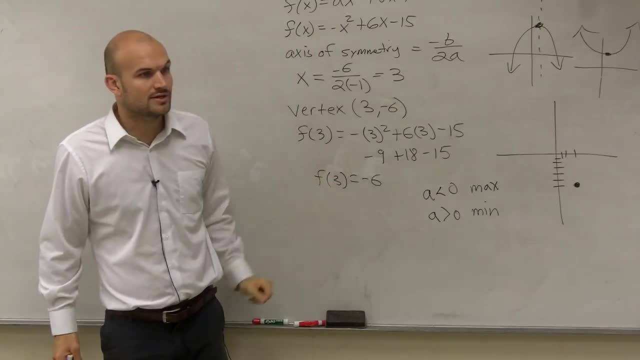 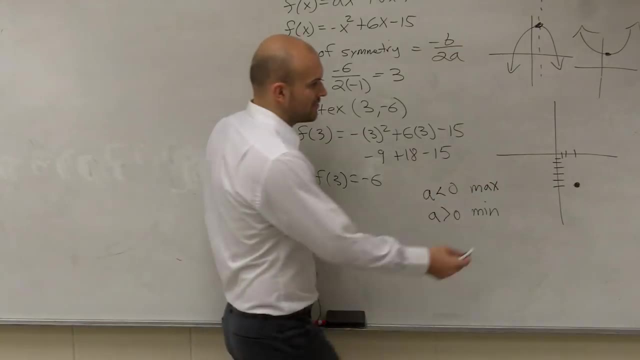 My A is negative, 1, correct. So is A greater than or less than Less than So. therefore, that means that's a maximum point, Right? So my graph's going to look something like this: All right, 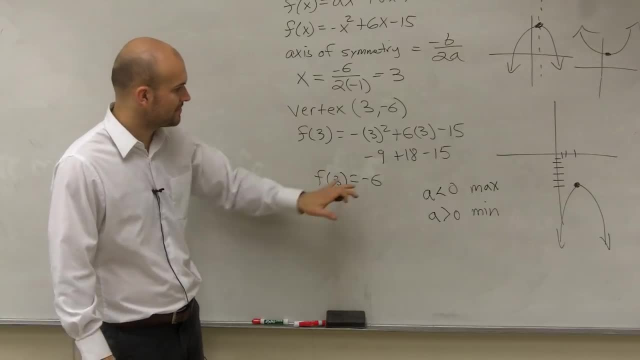 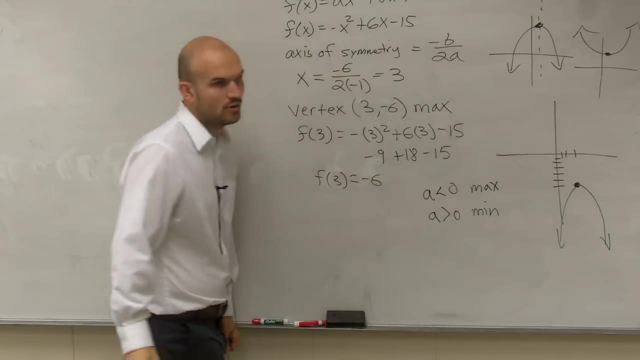 I'm just going to. we're not going to work on sketching right now. We'll do table values later. So my maximum point looks like that. So we could say that's my vertex, which is a maximum point. So that's what you guys should have wrote. 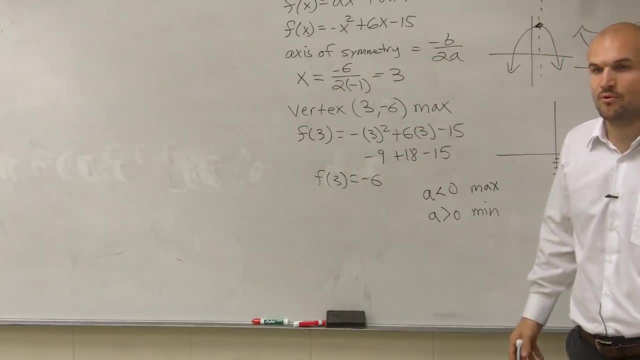 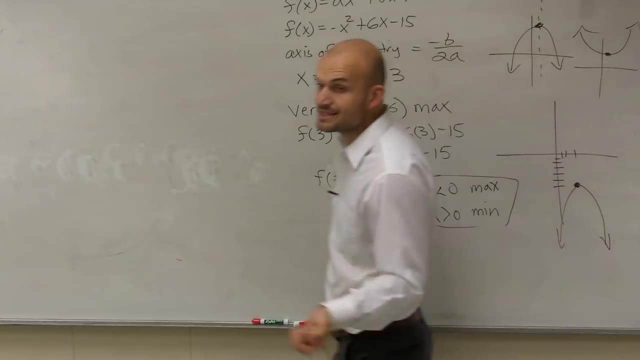 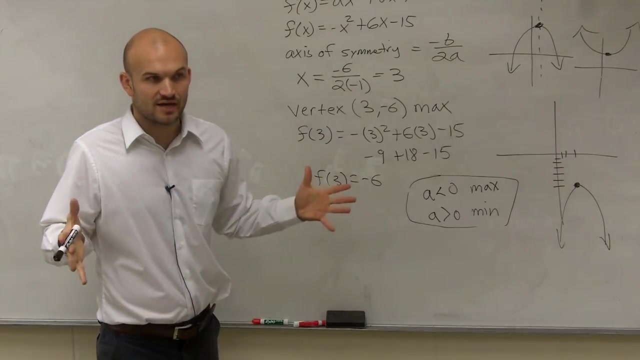 for your maximum point. That is my vertex, which is a maximum point Because the graph opens down because of this rule that we worked on Then. the next thing that got students very confused was the domain and range. Remember, the domain is the set of all X values. 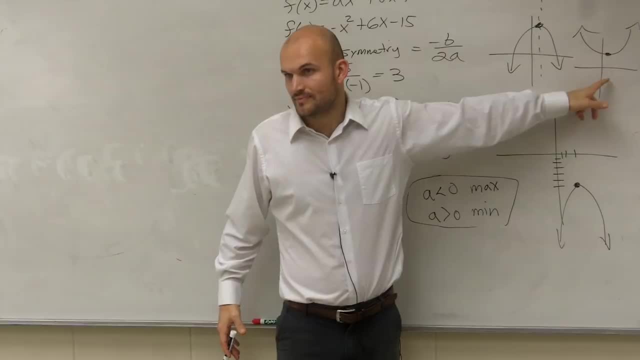 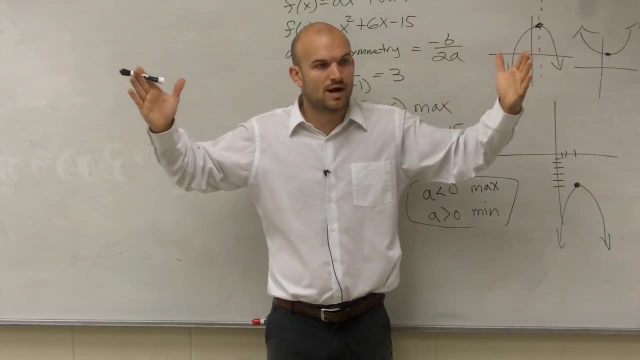 that are part of your graph. Ladies and gentlemen, look at these two parabolas, All right, And think about any parabola you've ever graphed or looked at. These parabolas are going to infinitely, just keep on getting wider and wider. 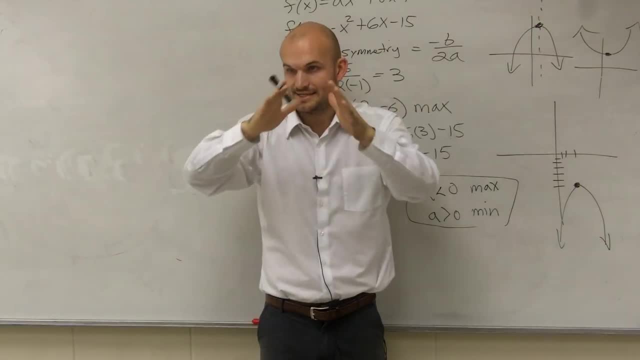 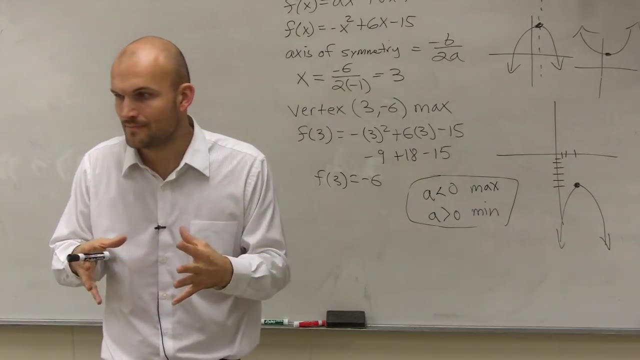 Right. As they go up, they're going to keep going. They're going to keep on expanding. As they go down, they just keep on getting wider. So eventually they are going to encompass every single X value that we have in the number system. 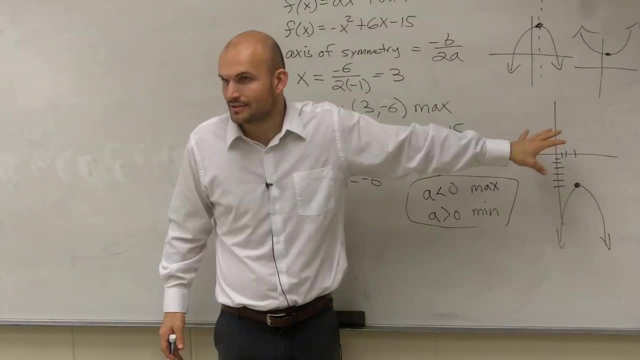 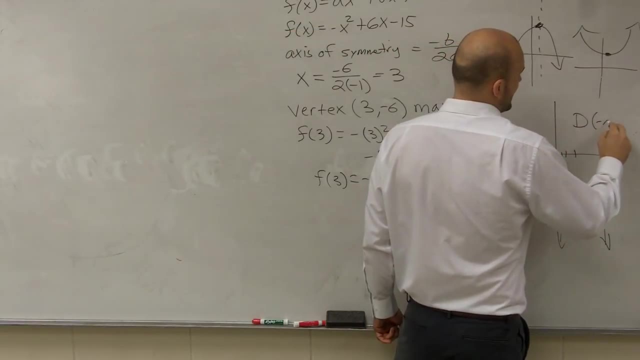 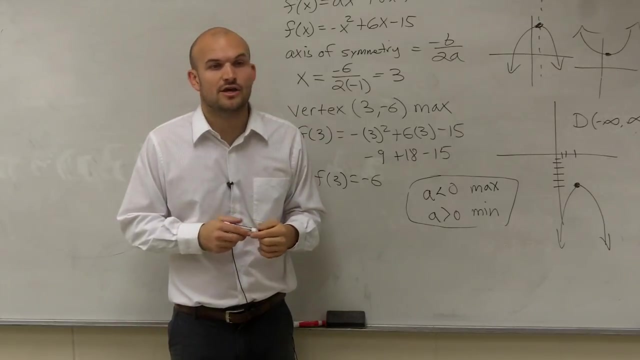 Every single one. So therefore, the domain for a quadratic without any constraints is going to be all real numbers. So your domain is going to go from negative infinity to infinity. Pick any value to be X. Emma, give me a value for X. 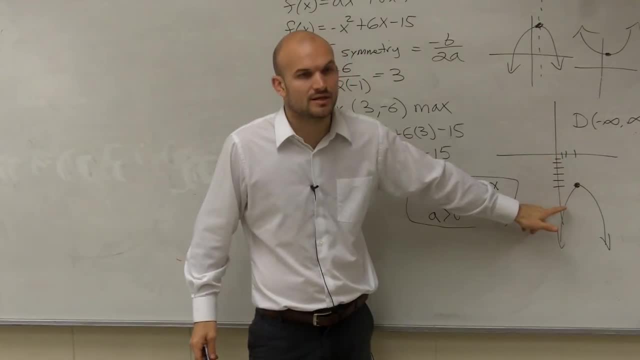 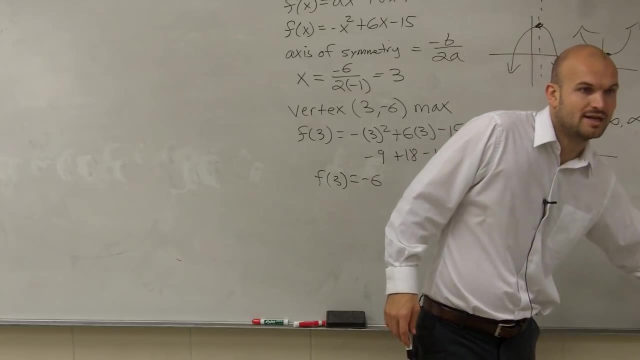 Two. Two Is two a value. Yes, It's right there. Give me another one, Eighteen. Eighteen Probably be over here, right, But when you go down, will this graph eventually have a coordinate at 18?? 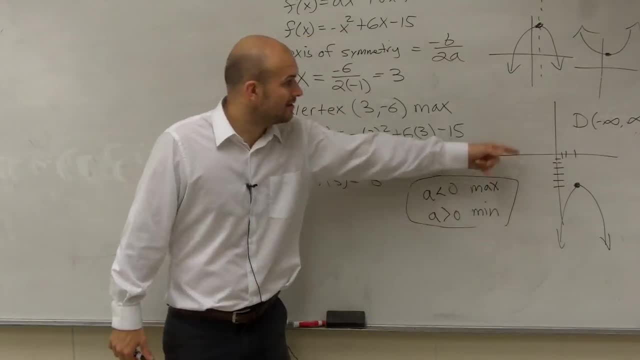 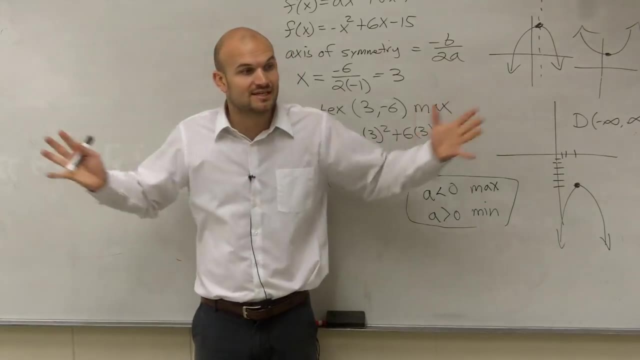 Yes, Right, And you can do negative 300.. Way over there, But it's still eventually all the way down there. eventually it's going to have a point Correct, Because these graphs keep on expanding. However, the range is going to be the Y values.